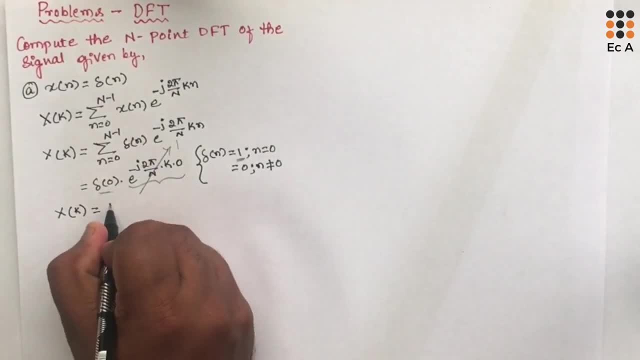 the DFT of given signal as 1.. Let us take the second problem, where the signal x of n is given as delta of n minus n naught, where n naught is equal to 1. So we will get the DFT of given signal. 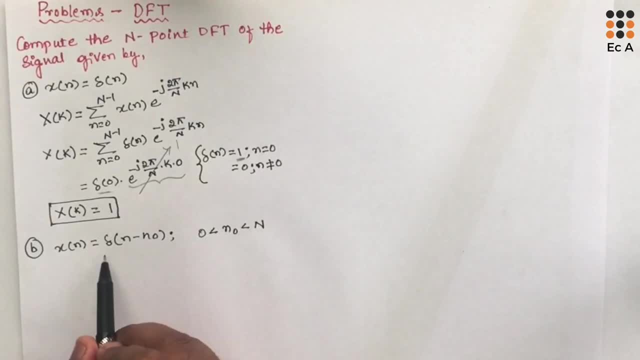 as delta of n minus n naught. Now let us write if any bets For any bets. if we have any bets, we have to be prepared for this. So we have to write the DFT of given signal. and here we have to ask what will happen to d for 0, 1, i is equal to delta. sorry, this dx, d, z is called x power to d of I. 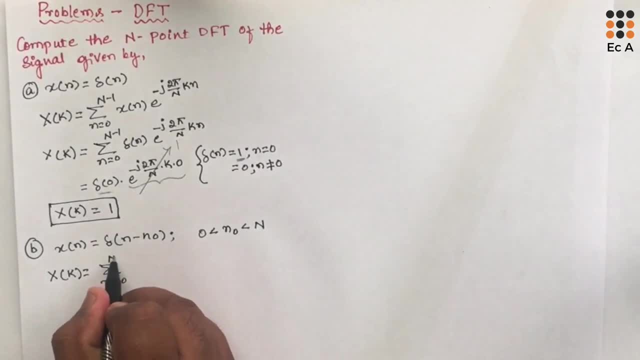 d z delta into d T. We will then be able to put the summation of delta of n, so the sum of delta of n is equal to Dj j Cos, delta of n minus bunn, equal to delta of e, by measured by delta our. so for this, everyone different set the value of d we have to take. 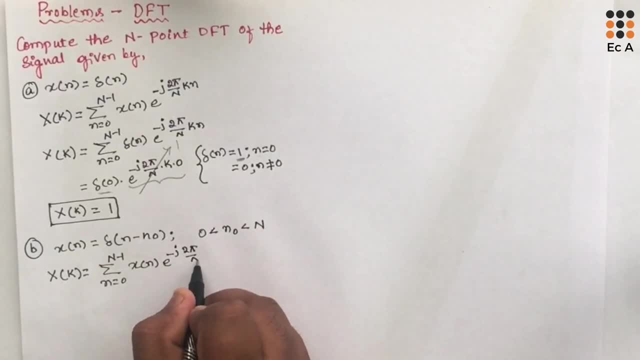 function of delta. So we will get: delta of n minus n is equal to 1.. For this flips of end to Labour power of n minus j b times very important. so we will take an extension of volts for one by d, t and so on. right, So we will come to this equation by as well. 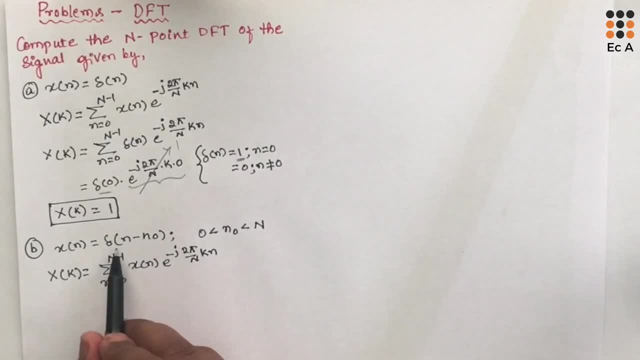 In this formula, let us substitute x of n as delta of n minus n naught. So we can write: summation of n is equal to 0 to n minus 1. delta of n minus n naught into e to the power of minus j. 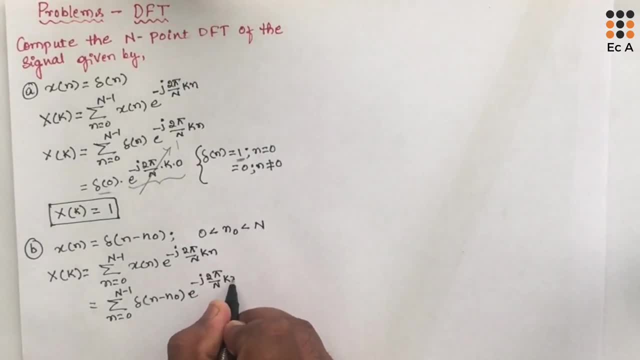 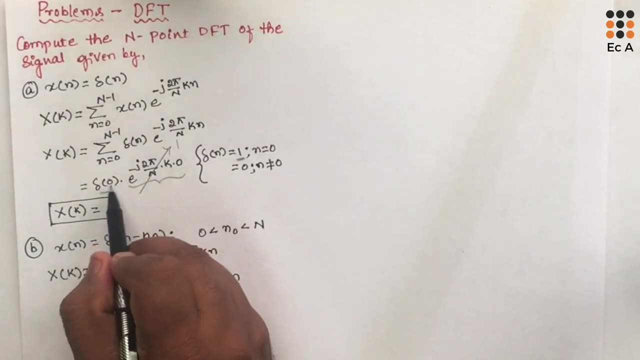 2 pi by n into k n. Similar to first problem in delta of n, when value of n became 0, this entire term become 1.. Using the same analysis, we can write: this term will become 1 when n minus n naught is equal to 0. So at that case we can say n is equal to n naught. 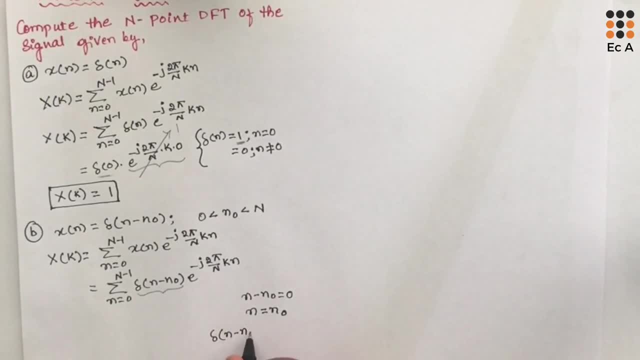 So we can write: delta of n minus n naught will be equal to 1 when n is equal to n naught and it will be equal to 0.. When n is not equal to n naught, So only when n is equal to n naught, this term will become 1.. 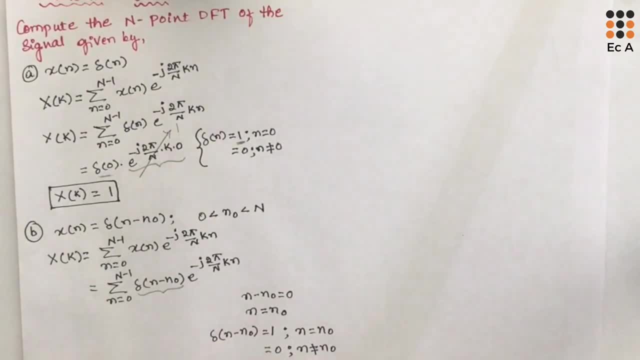 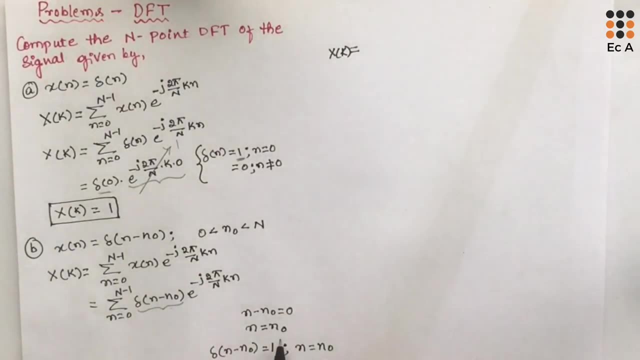 For other values, this term will become 0. So we can write: x of k is equal to this term. we can write 1 when n is equal to n naught, So it is 1 into e to the power of minus. 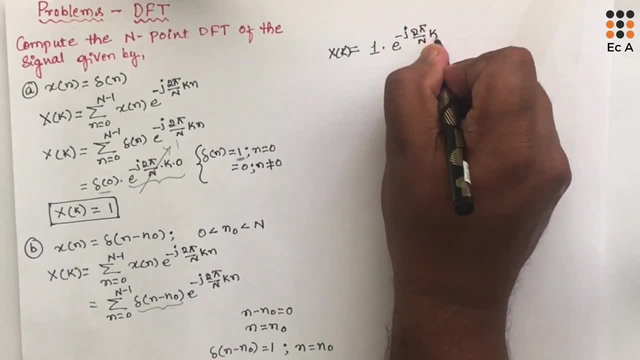 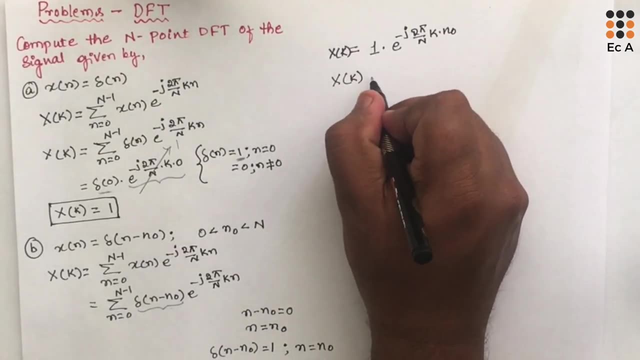 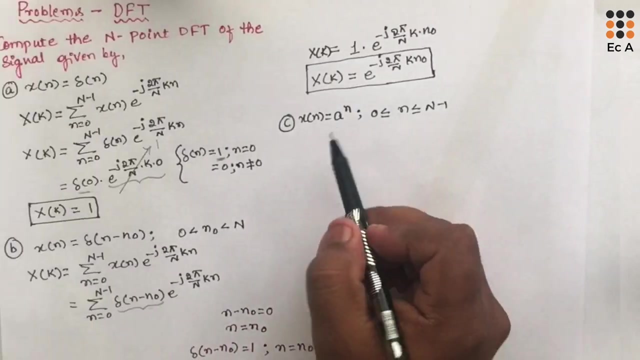 j 2 pi by n into k, into n naught. So the DFT of the given signal x of k is equal to e to the power of minus j 2 pi by n into k, n naught. Let us take the third problem, where the signal is given as x of n is equal to a to the power of n. 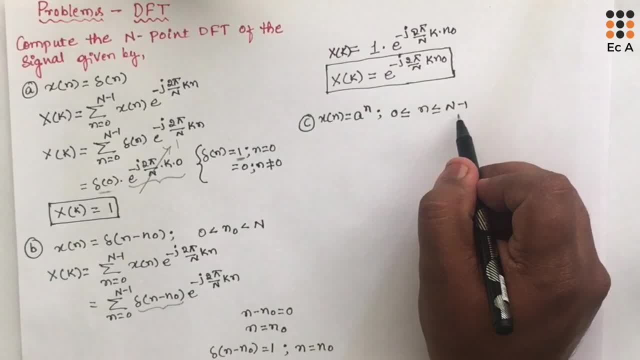 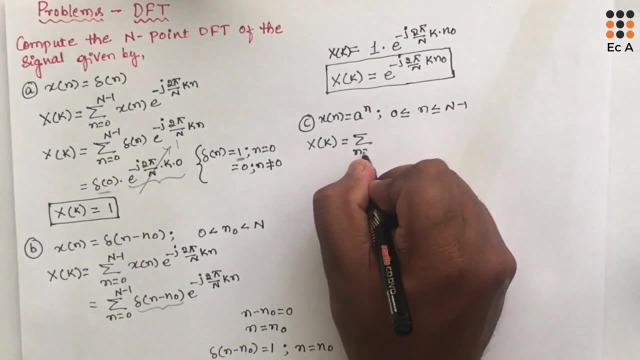 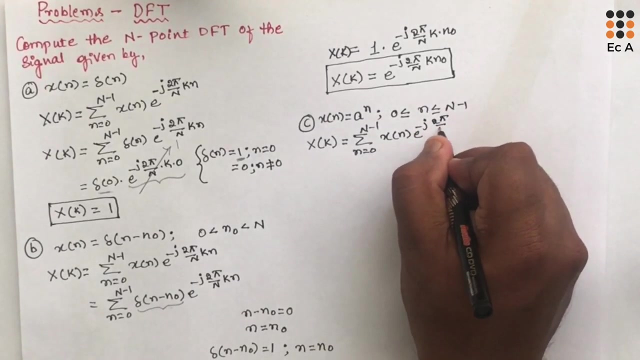 Here the value of n is ranging between 0 to n minus 1.. Let us write: the formula: x of k is equal to summation of n is equal to 0 to n minus 1. x of n, e to the power of minus j. 2 pi by n into k: n. 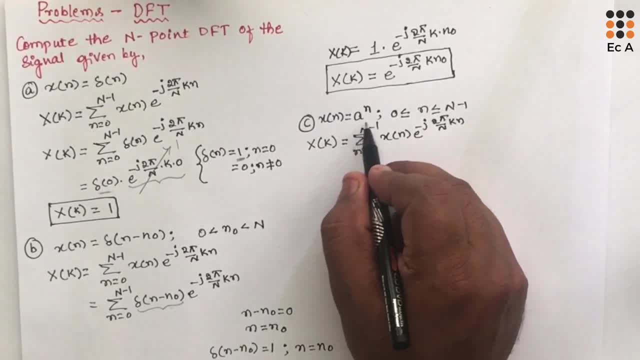 Let us substitute the value of x of n as a to the power of n, So in this formula we can write: summation of n is equal to 0 to n minus 1, a to the power of n, e to the power of minus j. 2 pi by n into k: n. 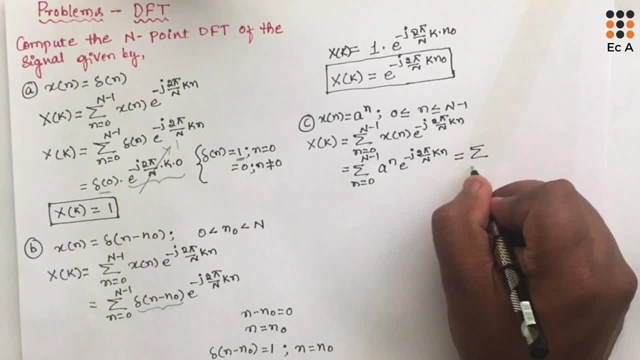 So this we can write it as: summation of n is equal to 0 to n minus 1.. If we take power of n as common in these two terms, we can write a into e to the power of minus j, 2 pi by n into k whole to the power of n. 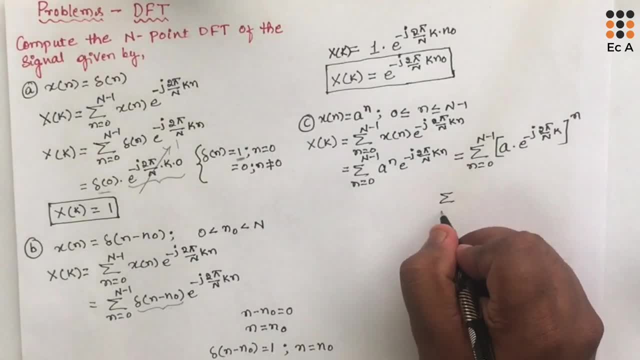 We have a formula which says: summation of n 1 to n 2, a to the power of n can be written As: a to the power of n 1 minus a to the power of n 2 plus 1, divided by 1 minus a for a value not equal to 1.. 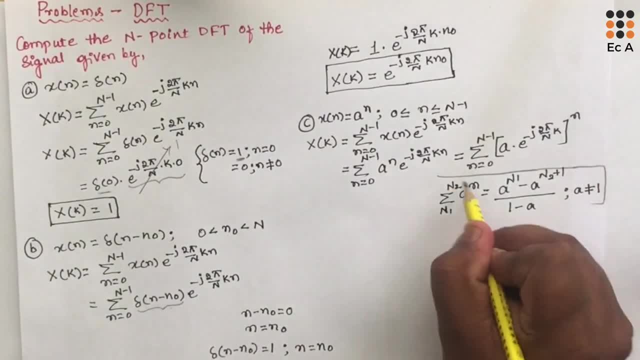 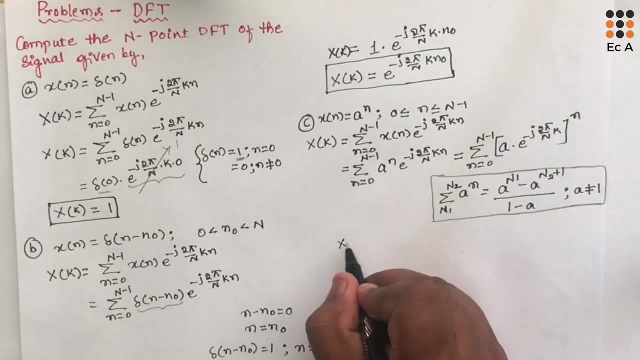 Remember this formula. This is very helpful for solving many problems. Using this formula, we can write the above expression as: x of k is equal to a to the power of n 1.. n? 1 is 0. So a to the power of n? 1 is equal to 1.. 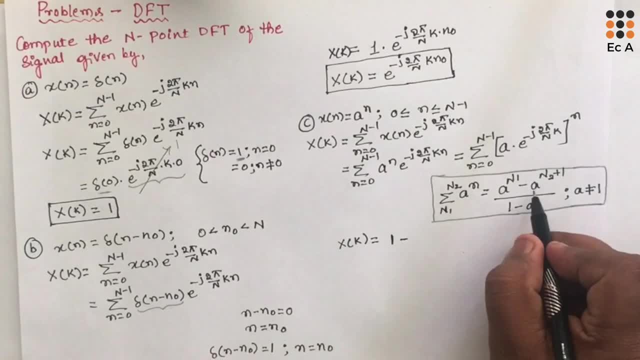 a to the power of 0, it will be 1 minus a to the power of n 2 plus 1.. n 2 is n minus 1.. So it is n minus 1 plus 1.. So plus 1 and minus 1 will cancel out.